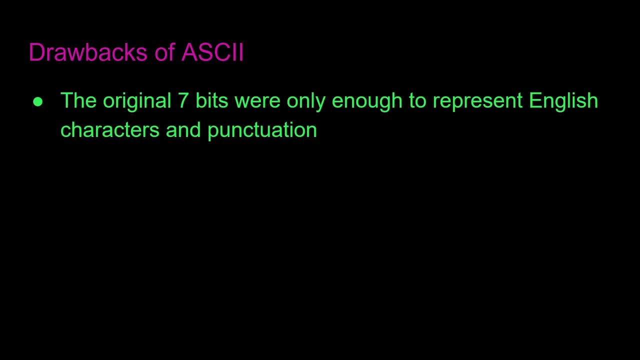 of ASCII. The original seven bits were only enough to represent English characters and punctuation and maybe some codes. And because a byte is eight bits there was a lot of competition on which other characters should be supported with that last bit Now enter Unicode. Unicode is a universal character encoding. It supports many different. 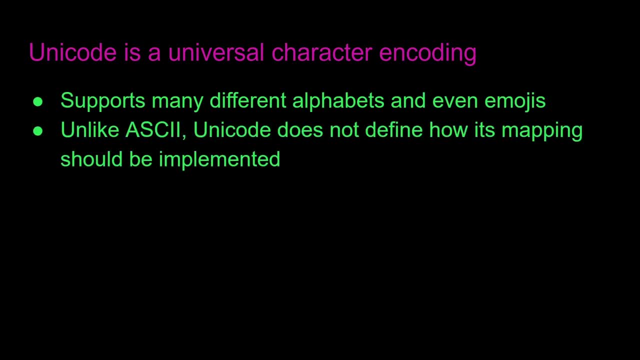 alphabets and even emojis. However, unlike ASCII, Unicode does not define how its mapping should be implemented, And we'll get into the details of that in a little bit. It only specifies which character refers to which code point, And a code point is a hexadecimal number representing a 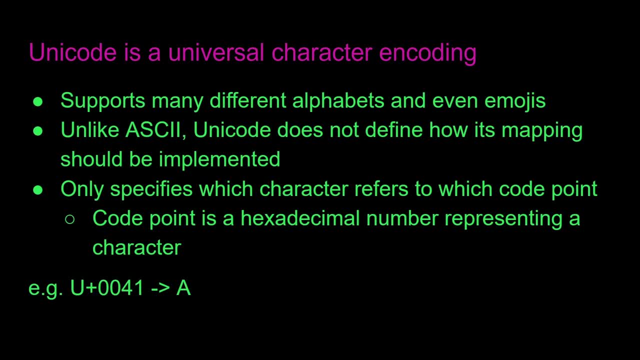 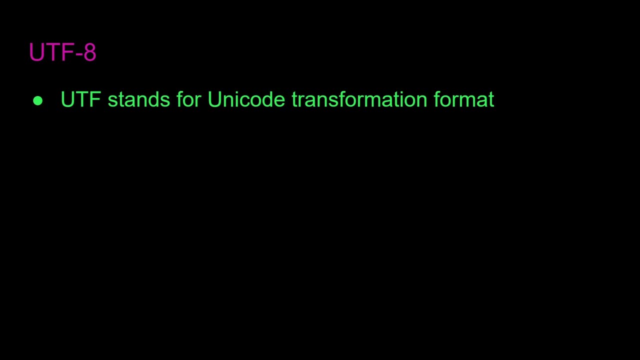 character, For example, U plus 0041.. Note that that's hexadecimal, represents A And 0041. hexadecimal is actually equal to 65 in decimal. Now enter UTF-8.. UTF stands for Unicode Transformation Format. It is an algorithmic. 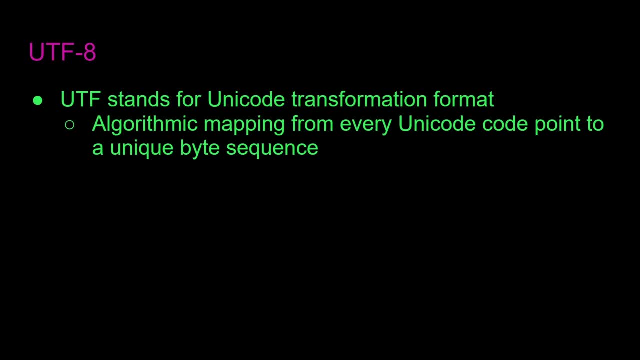 mapping from every Unicode code point to a unique byte sequence. UTF-8 is nice because it has variable length encoding. This means characters with code points with small values, like A, can be represented with just one byte, And characters with code points with large values. 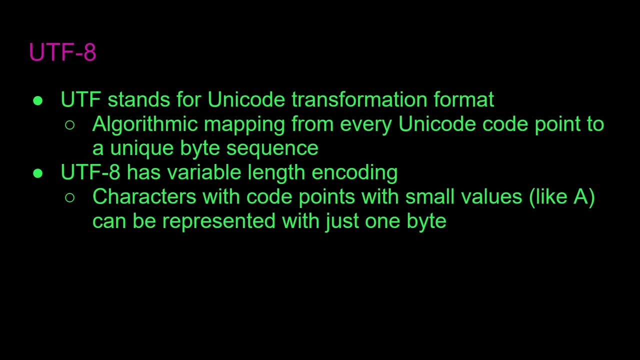 can be represented with more bytes as needed, And it goes up to four bytes. Another nice property of UTF-8 is that it's backwards compatible with ASCII. This means that any ASCII file can also be read with UTF-8.. Note that this is true with UTF-32 as well. 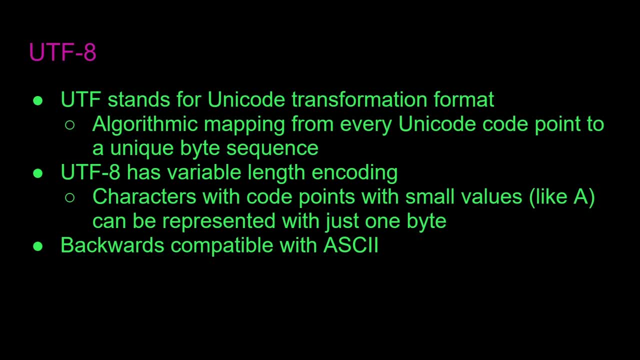 but not for UTF-16. But we won't get into that here. Because of these two nice features, UTF-8 is now the most popular UTF-8 file in the world, And it's also the most popular UTF-8 file in the. 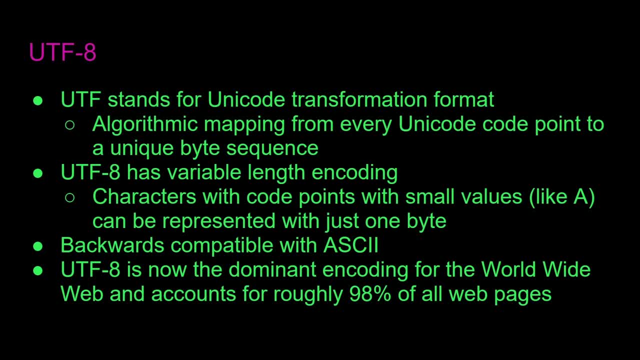 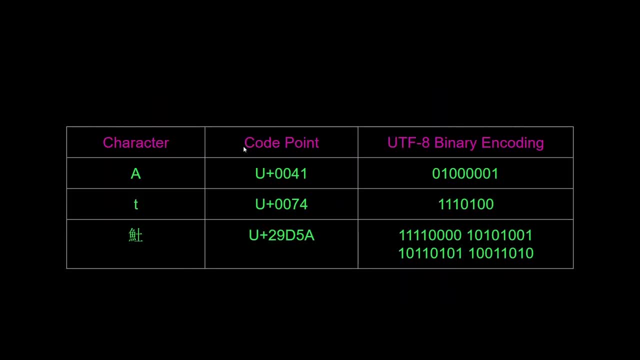 most dominant encoding for the world wide web And accounts for roughly 98% of all web pages. So we can see here the characters on the left, the code points in the middle and the UTF-8 binary encodings on the right. We can see that the character A has a code point of U plus 0041.. 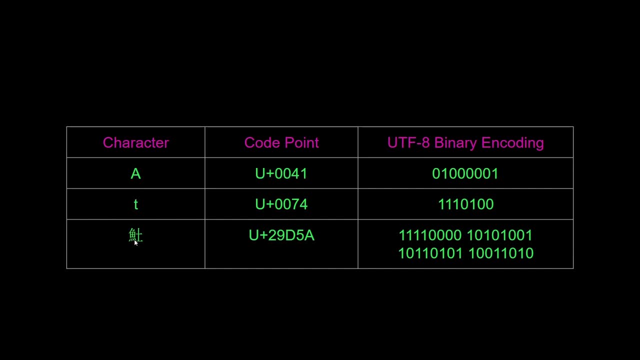 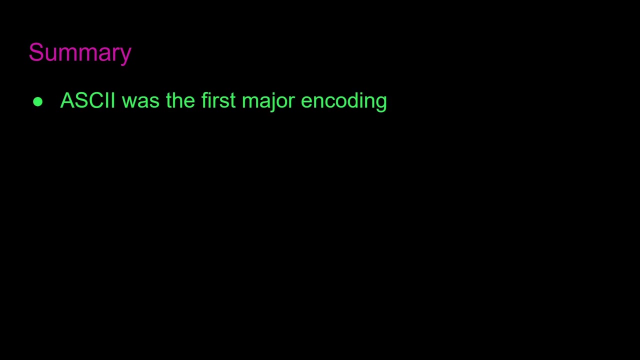 Note that's hexadecimal, And here is the binary encoding. Now this is a Chinese character on the very bottom. It has a much larger code point. This is a much larger hex value And therefore it needs more bytes to be represented in binary. So here's a summary. ASCII was the first major encoding.